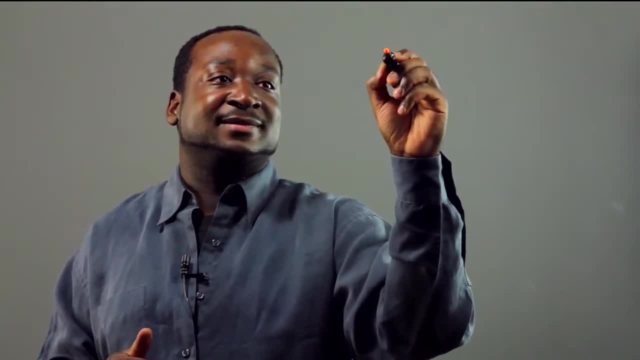 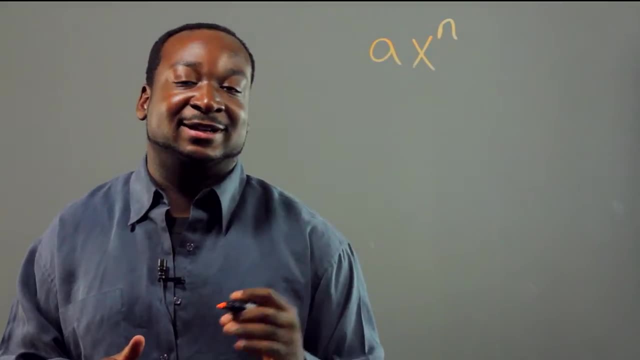 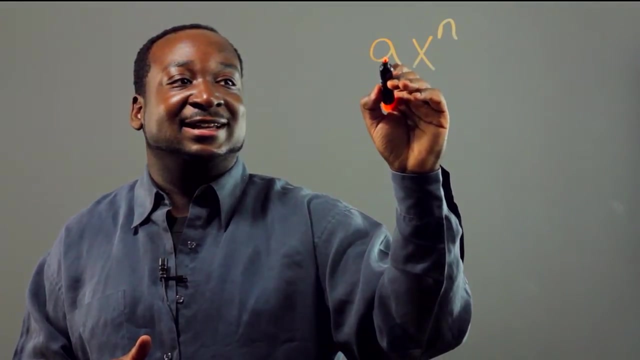 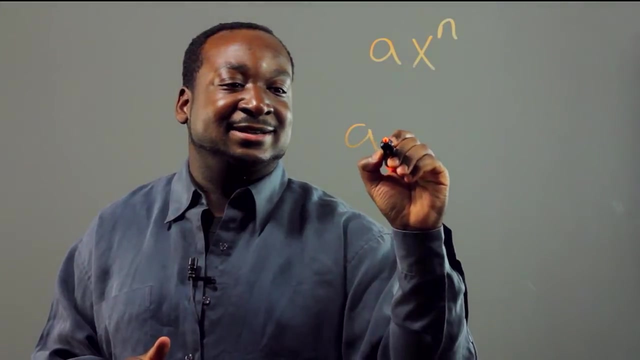 Let's say we have the term- here's a general one- a times x to the n. There's a general term here. I'm going to show you how to take the derivative of this. What do you do is multiply a, which is the coefficient times the exponent. so that's a times n, Add x there. 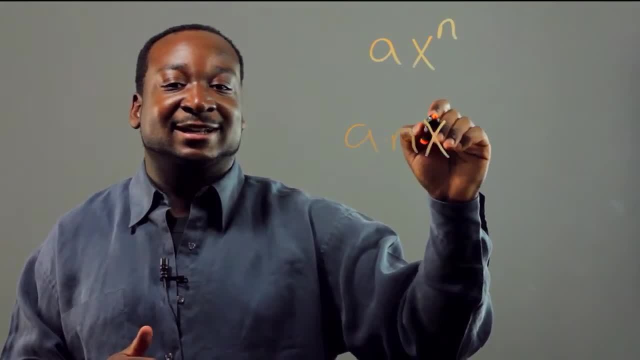 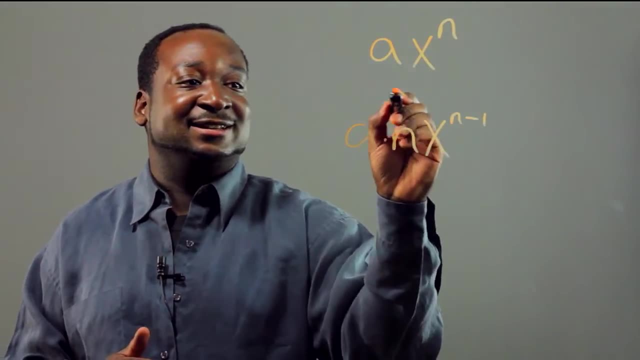 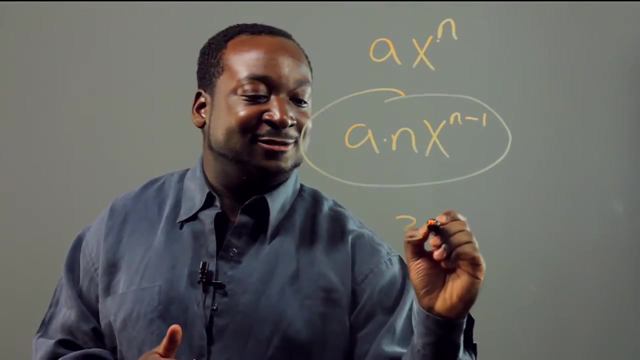 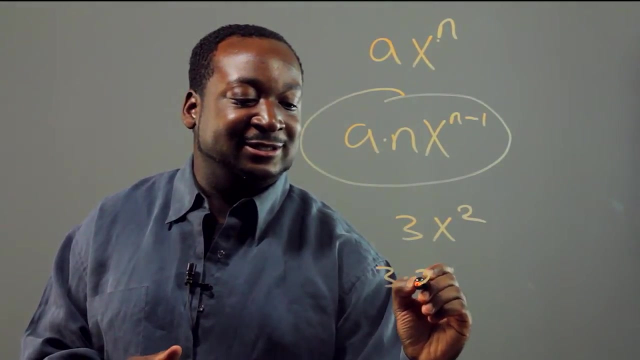 and you're going to keep the same exponent and subtract it by one N minus one. Here's the derivative of this. Now, let's apply it. Let's take three x squared: That's going to be three times two multiplied by x. 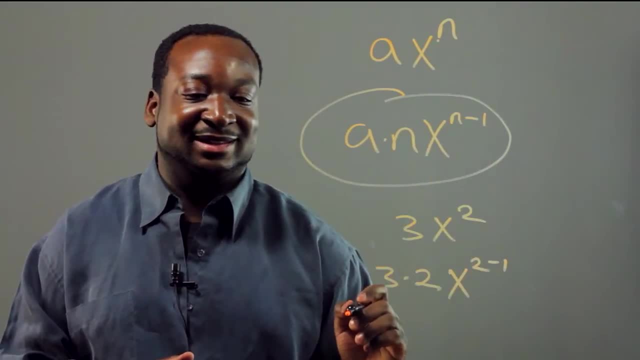 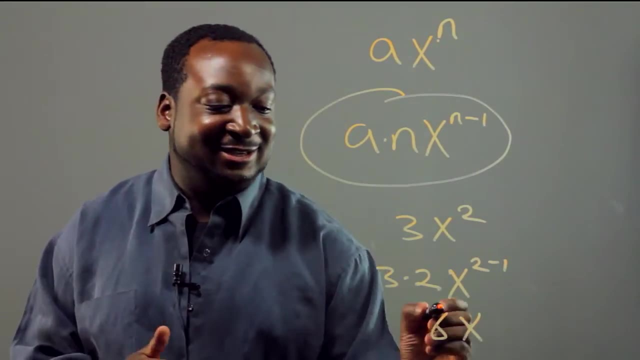 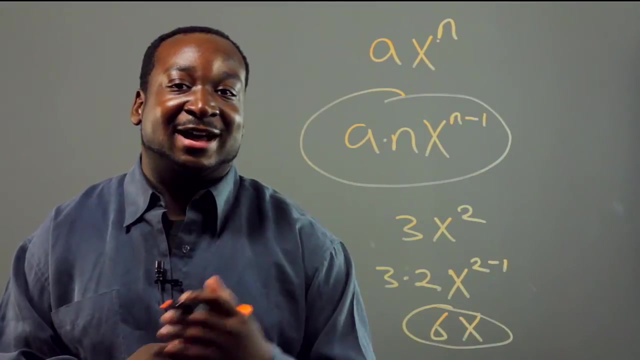 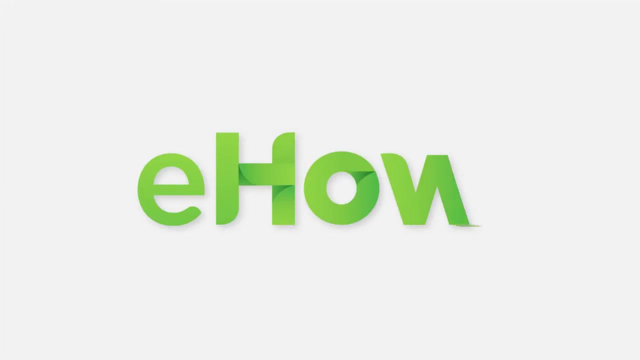 Two minus one, Basically you get six x. Here's our answer. That's the derivative Great, That's simple ways of how to take a derivative and that's some basic calculus. Thank you.